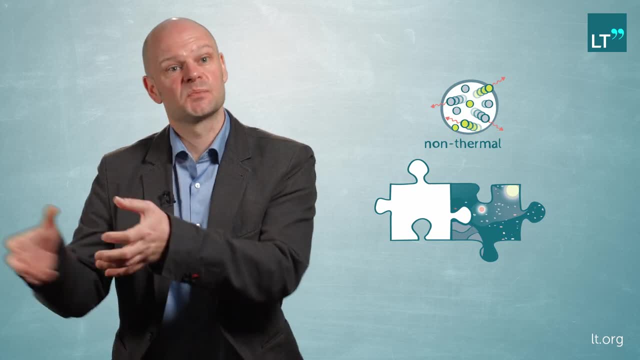 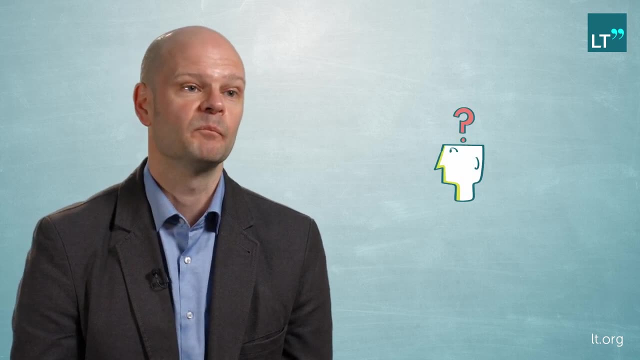 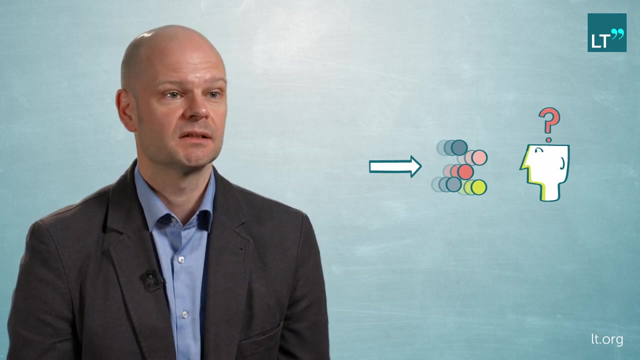 until we can really put this aspect of astrophysics on the same footing as thermal astrophysics. The big question is: by what processes are these particles being accelerated? Where And then what do they do? What is their impact? And potentially then, by looking at the universe and these high energies, 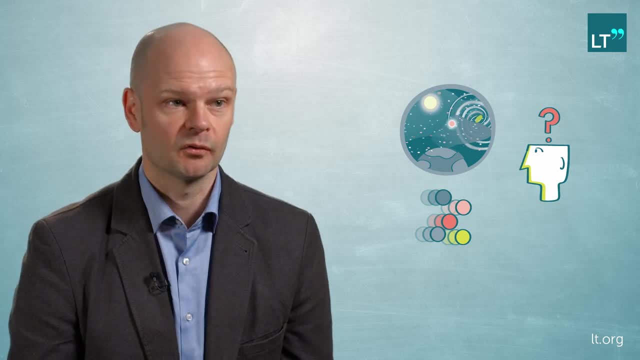 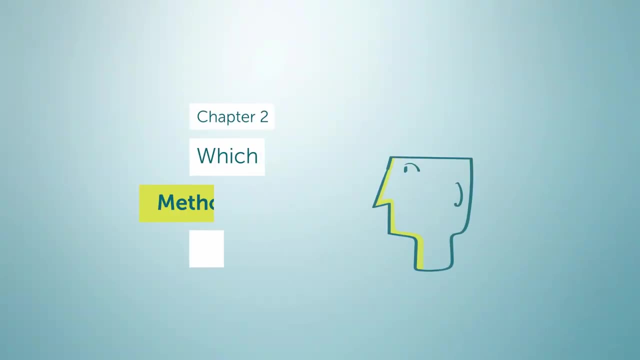 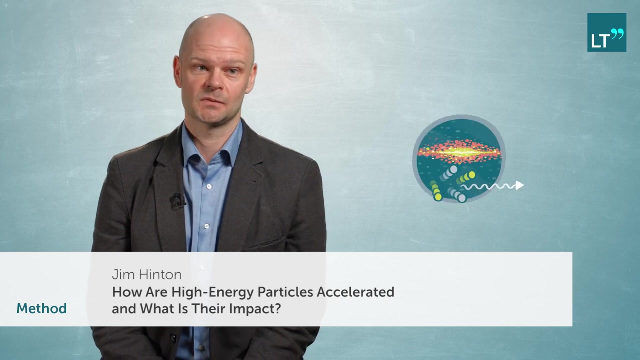 we can find out, get a completely new perspective on the way the universe works, and may have to rethink many, many things. The method we use is to look for very high energy gamma rays. So these gamma rays are produced in the interactions of accelerated charged particles. 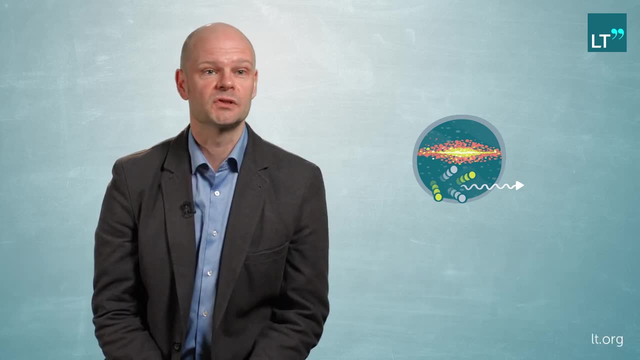 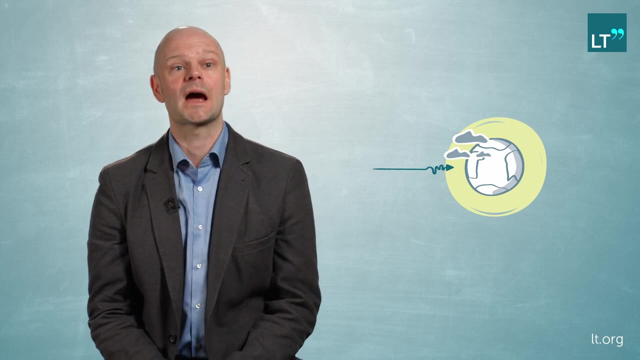 and travel in straight lines towards the Earth. Now, gamma rays- luckily for us, don't reach the surface of the Earth. They interact in the Earth's atmosphere And for low energy gamma rays this means they're basically absorbed and they're gone. 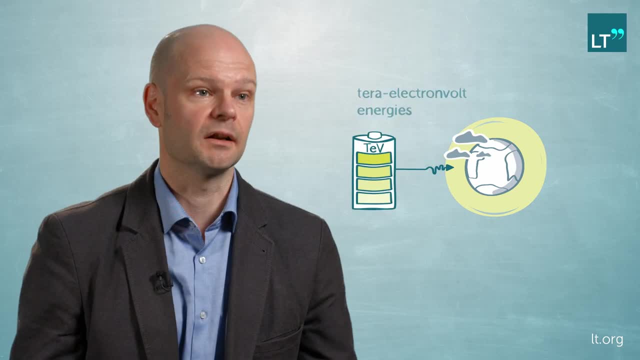 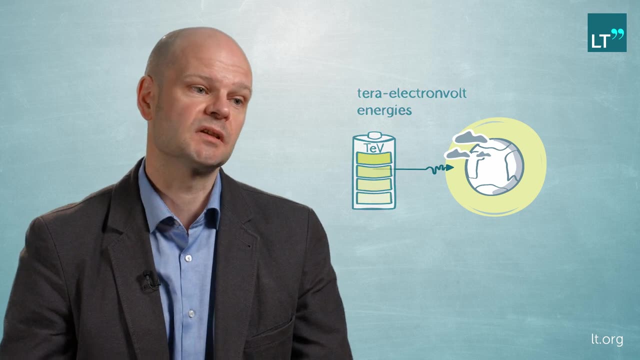 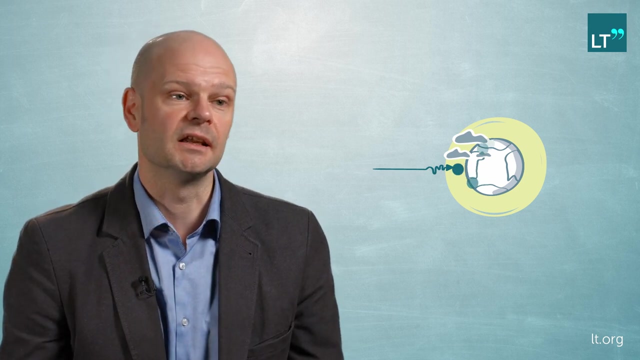 But at these tera-electron volt energies. we're talking about photons that are a billion times more energetic than X-rays. what happens is that the interaction of the gamma ray produces a cascade of particles in the Earth's atmosphere, And then individual particles in this cascade can be traveling faster than the speed of light. 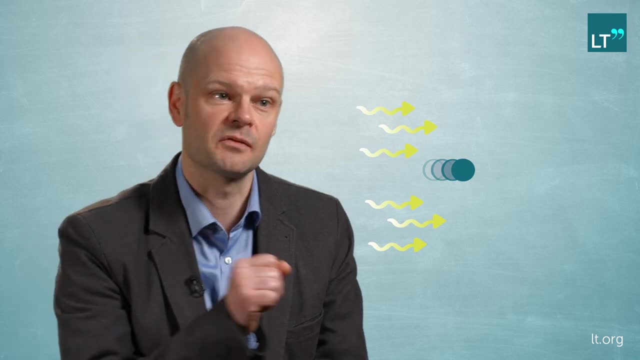 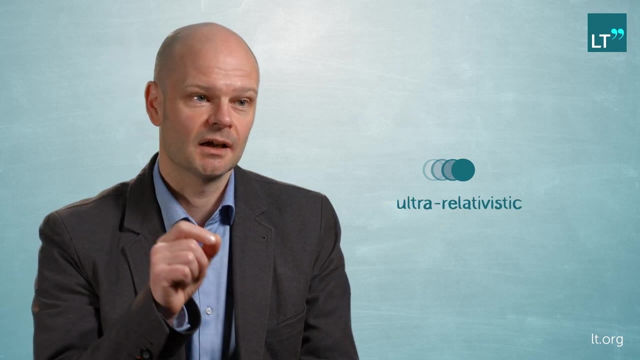 Of course this sounds implausible, but this is faster than the speed of light in air, which is a little bit slower than the speed of light in a vacuum. So these are particles that are ultra-relativistic and they go faster than light in air. 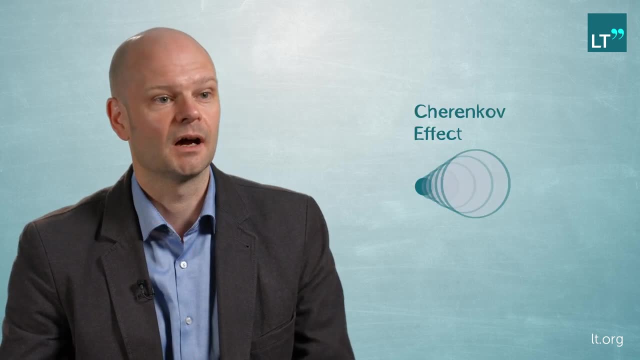 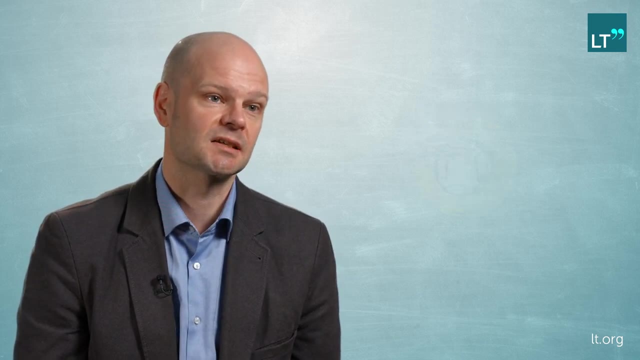 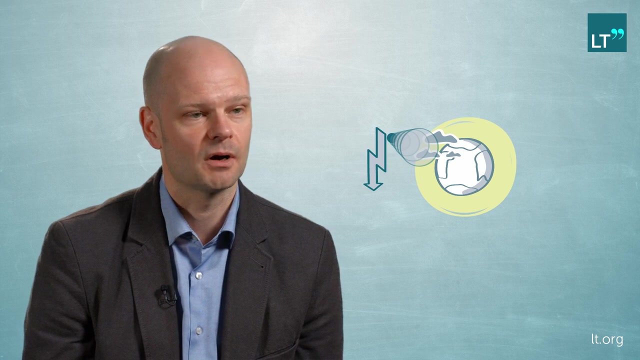 And then there is an effect called the Cherenkov effect which is basically producing a blue light, so in the optical band, And these cascades of particles therefore make a flash of blue light which is beamed in the direction of the shower. 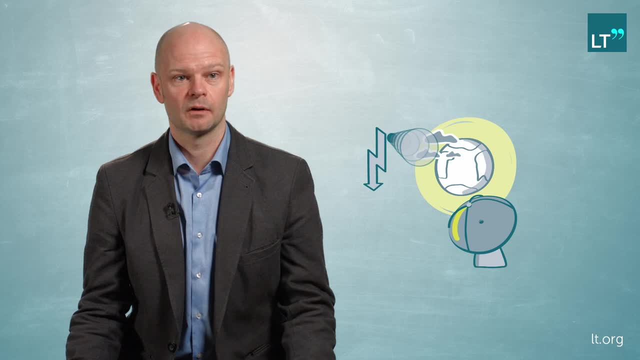 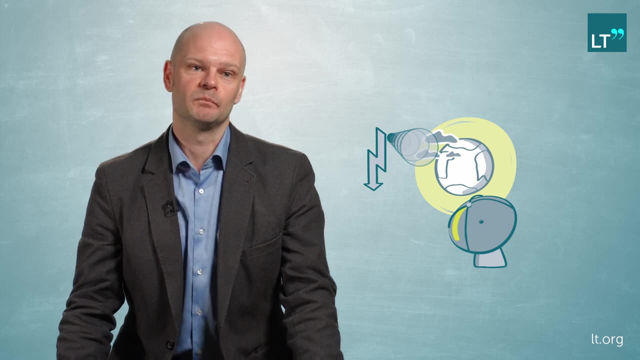 And if you put a very, very sensitive telescope on the ground and look for a few nanosecond long, a flash of light, a few billionths of a second, you can detect these gamma rays. And if we have several different telescopes all looking from different directions, 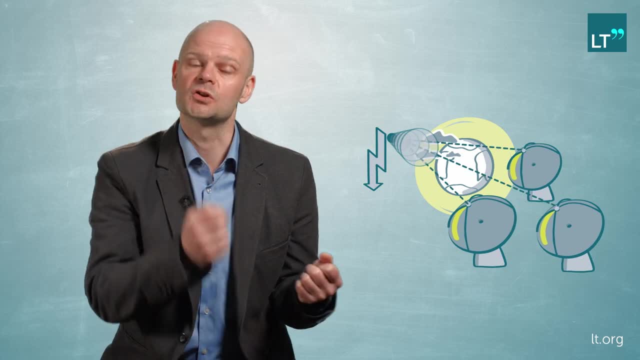 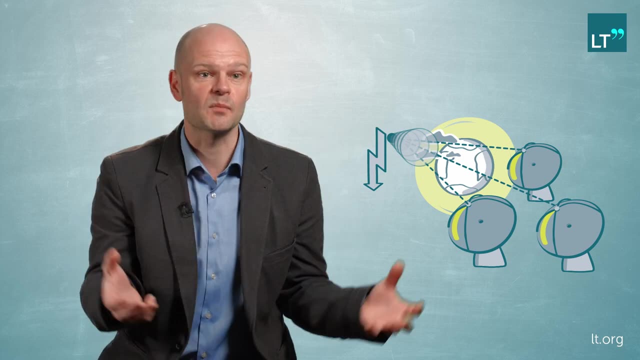 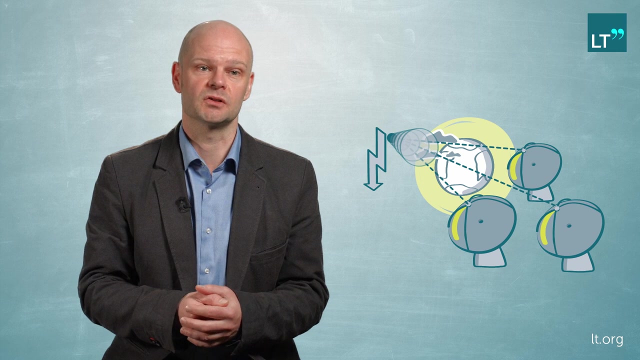 we can very well reconstruct the direction from which the original gamma ray came. So it's a very indirect way, if you like. We use the whole atmosphere of the Earth as part of our gamma ray detector. We use these many views of the shower from different directions. 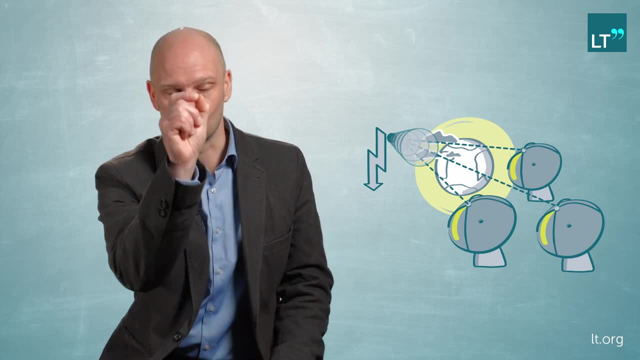 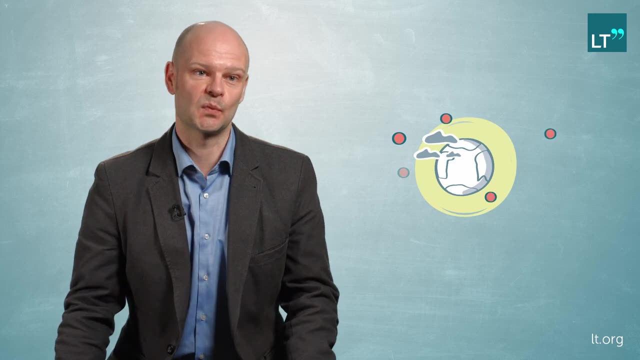 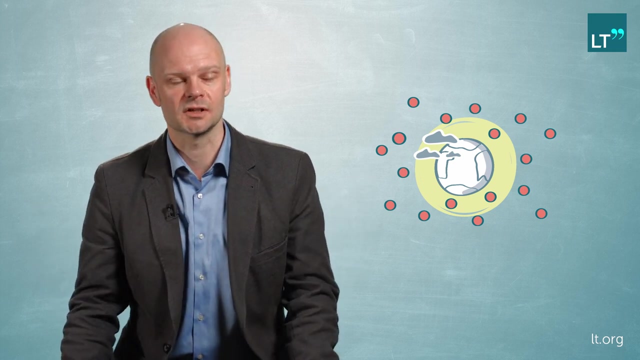 to reconstruct the direction of the individual gamma ray. And then we have one little point on our gamma ray map of the sky And then we collect many thousands of such events per second And over time we build up a view of what the high-energy sky looks like. 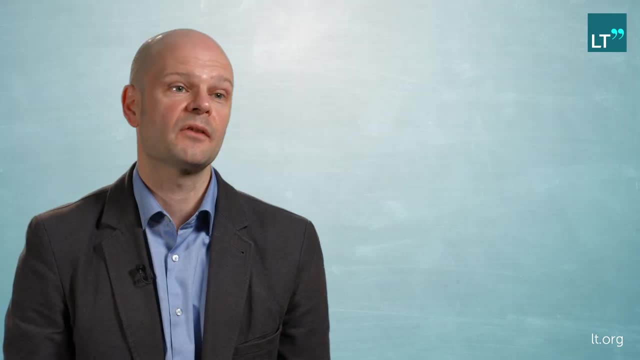 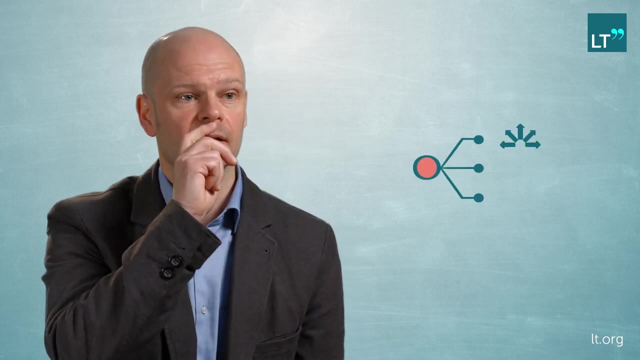 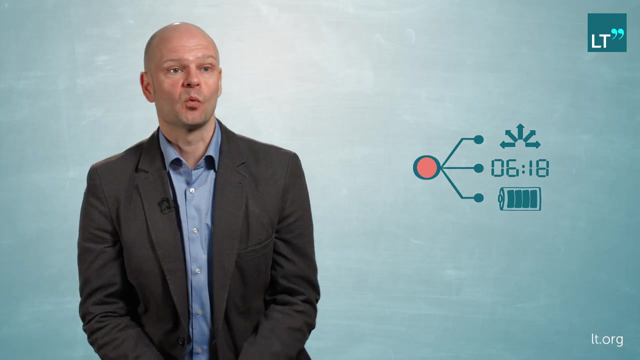 in this tera-electron volt domain. When we have recorded individual gamma rays, we reconstruct their direction and their arrival time and their energy. From the cascade we can calculate the energy of each individual photon. So then, what we can do is make a map. 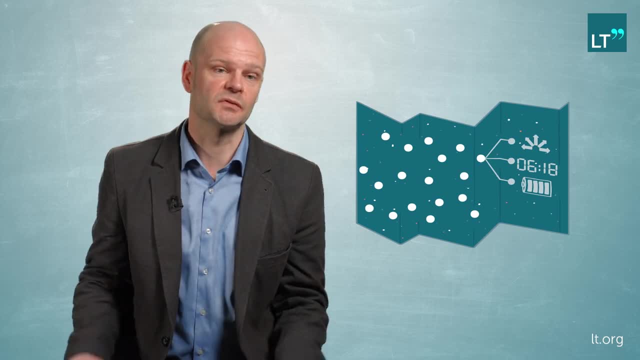 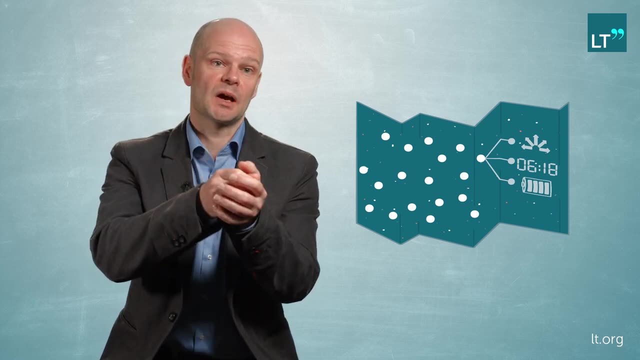 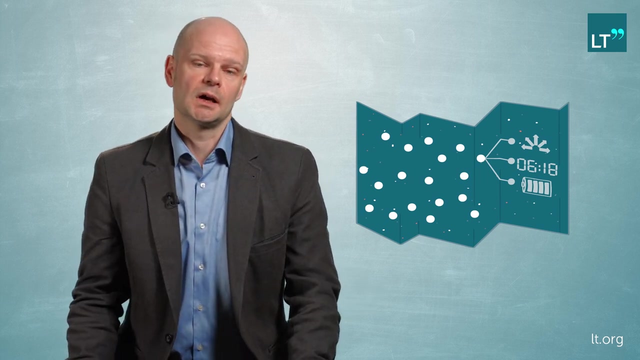 an image of the whole sky or parts of the sky that we survey, And then we will see individual sources of gamma rays, And for each source we can make the spectrum of gamma rays. We know the energy distribution, And so, by exploring the morphology, 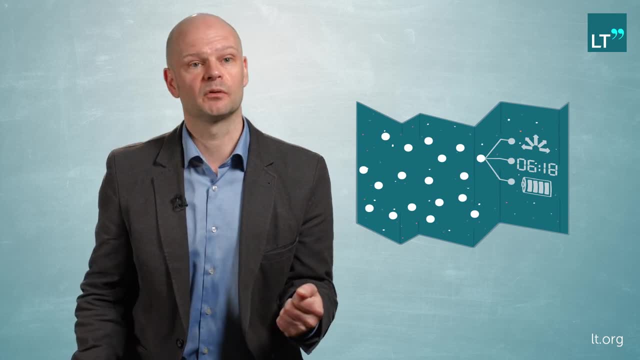 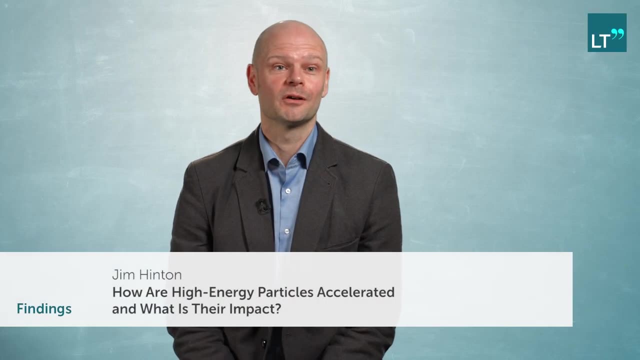 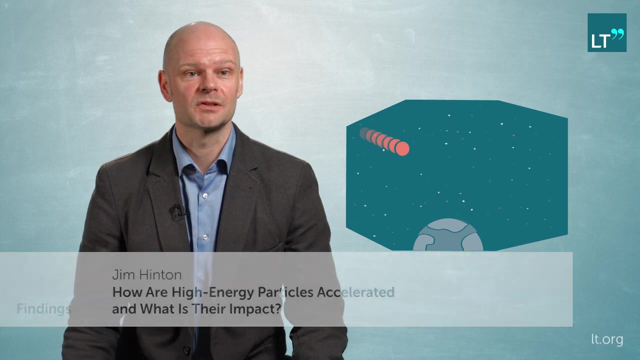 in the spectrum of the gamma emission from these sources, we can learn something about the way that they are accelerated. What we find when we look at the universe in these tera-electron photons is that the process of acceleration of particles to these extreme energies. 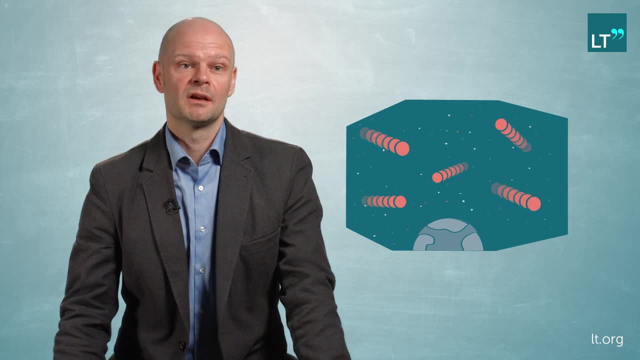 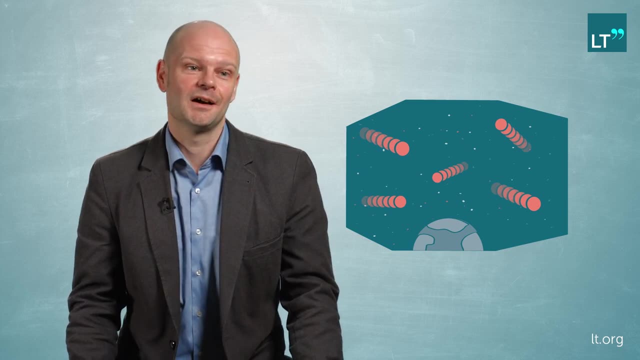 seems actually to be rather common in nature. So originally people thought, well, there will be one particular special source of these cosmic rays that we see at the Earth, And people thought probably supernova explosions. And indeed we see the shells of supernova explosions. 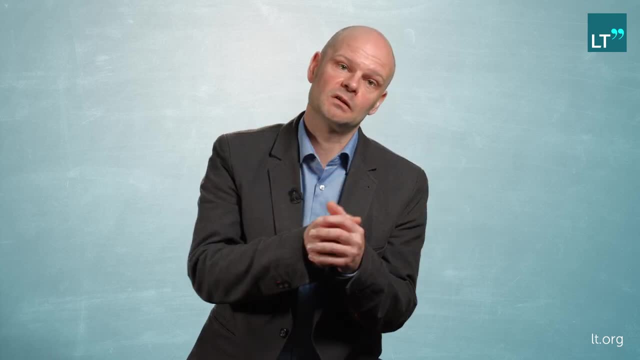 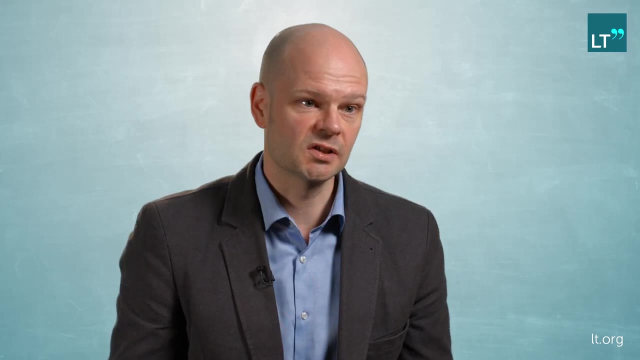 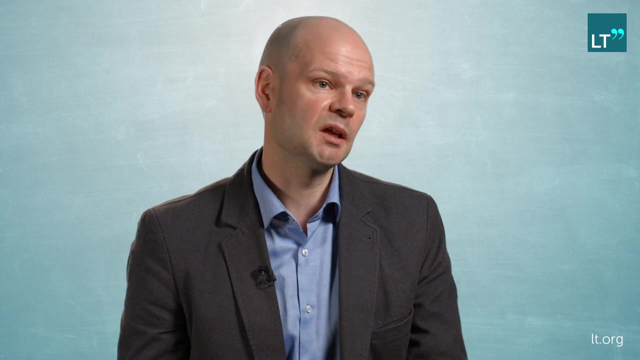 We see that in these blast waves, expanding shells around supernova, explosions, that particles are being accelerated unambiguously. But we see many other things as well. So the universe seems to be able to play this trick of particle acceleration in many, many places. It's not a sort of strange and unusual phenomenon. It's a normal astrophysical process. So we see this in the colliding winds from stars, the winds blown by stars. We see it close to pulsars and in the nebulae around pulsars. 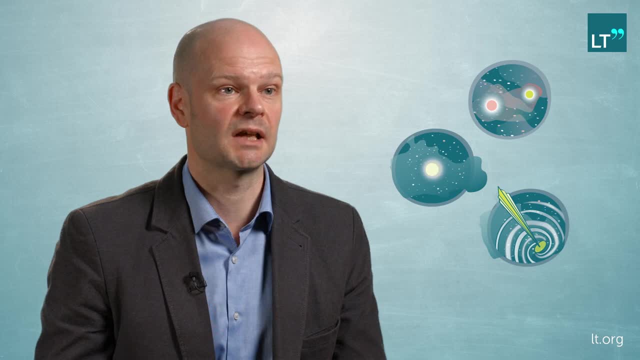 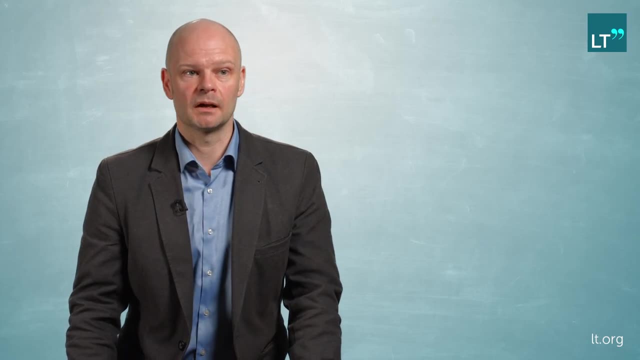 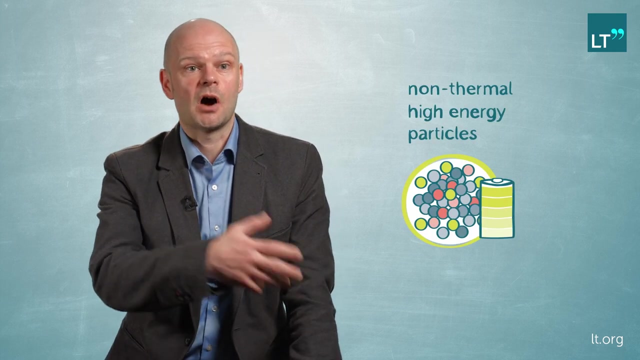 in the jets of active galaxies and emission around stellar clusters. So it seems that this is something we can't ignore, that these non-thermal particles, particles with an unfair share of the energy, are everywhere in astrophysics And we really now have to try and understand. 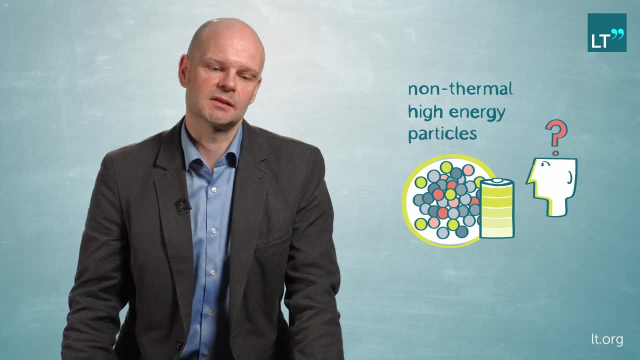 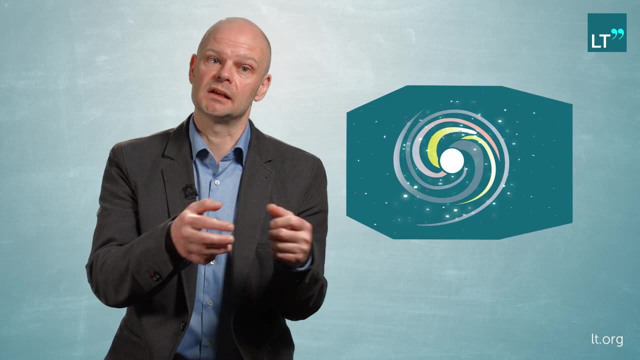 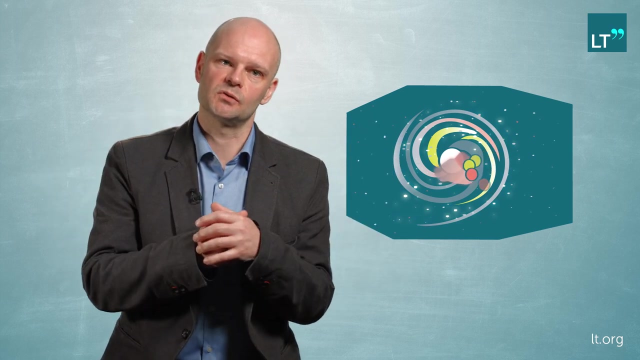 what they're doing there, what their impact is, And one recent example is the discovery that in the very central part of our own galaxy, in the so-called central molecular zone, we have diffuse gamma-ray emission from all of the molecular clouds that we see. 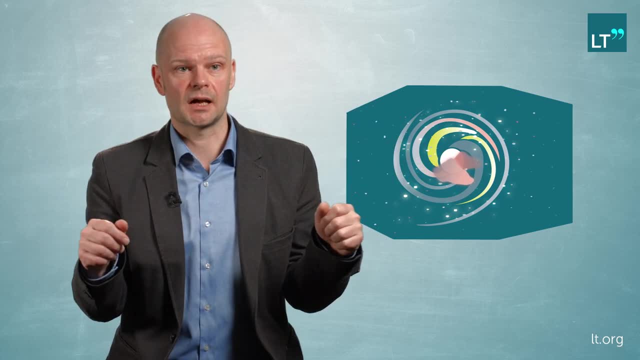 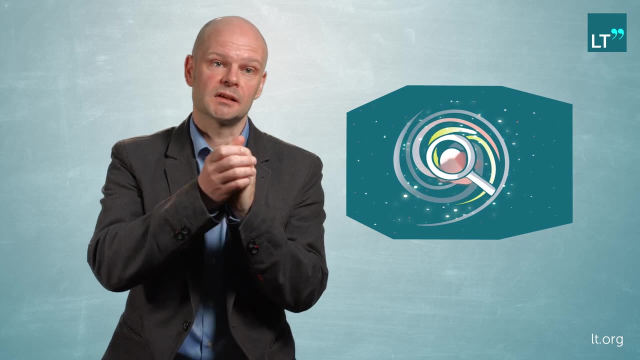 And from this gamma-ray glow of these clouds we can infer the density of relativistic particles, And we see that it can be done. It peaks at the very center of our galaxy. The profile is consistent with a diffusion of particles away from a source. 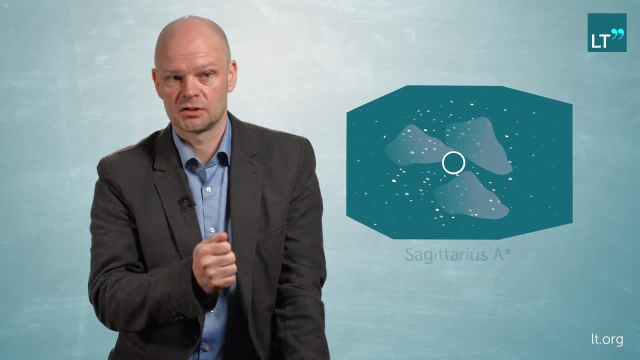 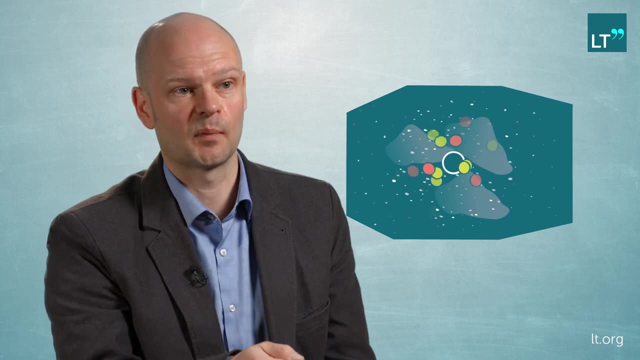 which is basically at the position of the supermassive black hole Sagittarius A star, And furthermore, the spectrum of the gamma rays indicates that particles are being accelerated close to the supermassive black hole to PV energies: 1,000 tera-electron volts. 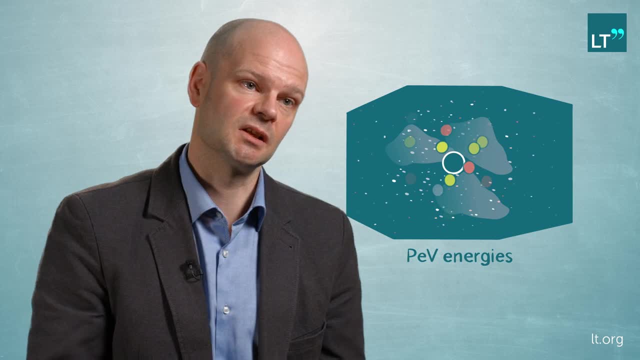 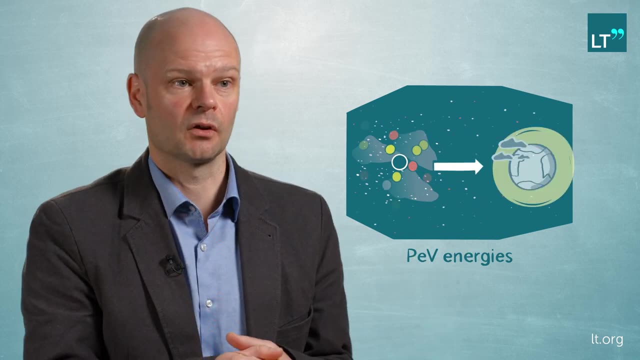 And this was really unexpected. So, in fact, this is the only place in the galaxy where we see acceleration up to these energies, And it could be that all of the PV particles we see at the Earth are actually accelerated at the supermassive black hole. 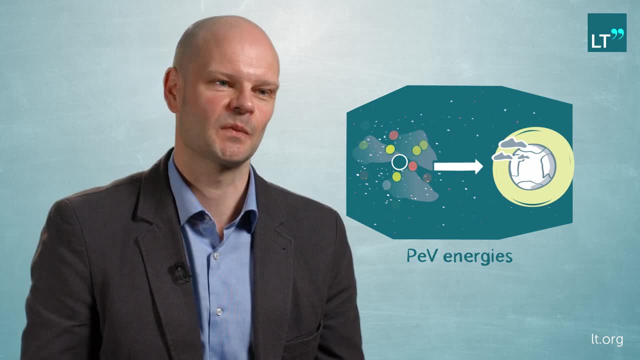 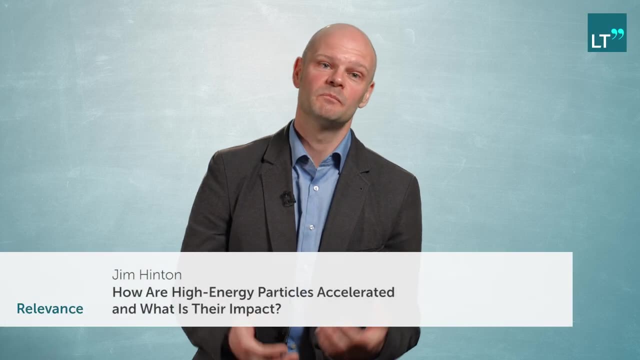 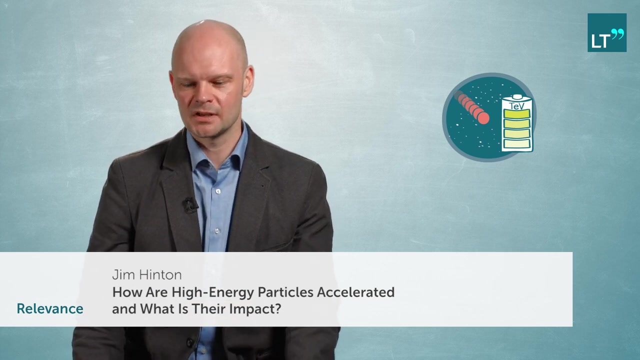 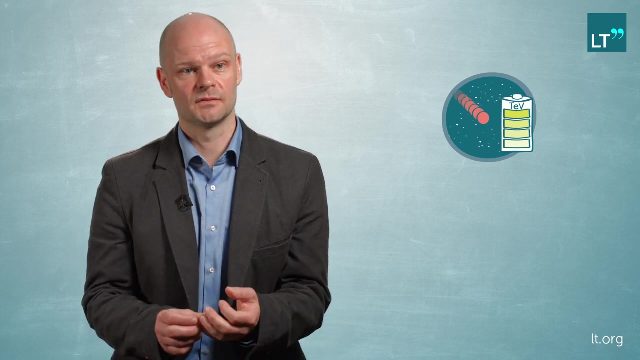 which is really against the conventional wisdom. We have for the first time now, a real picture of what is happening at TV- energies in the cosmos, And there is, from this clear experimental picture, a growing appreciation of the importance of these relativistic particles in astrophysical environments. So for many years there weren't good measurements And it was very difficult for people, you know, in their cosmological models or their models of the way that astrophysical systems evolved, it was very easy for them to ignore these things. 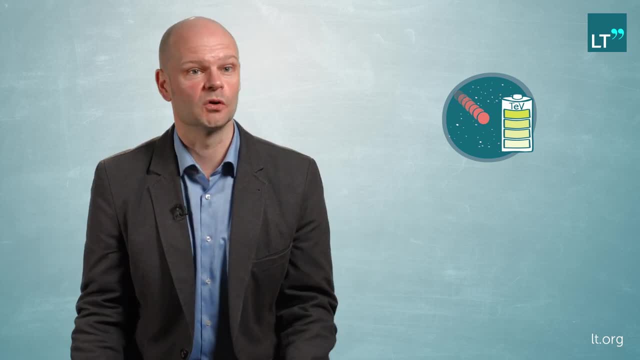 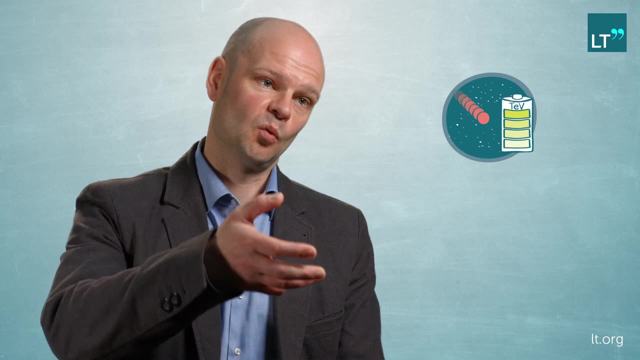 or very difficult if they actually wanted to include them, because there were no good data. So now I think people don't feel like they can ignore these relativistic particles anymore. So, for example, there's a study that shows that recent simulations of the way that galaxies evolve 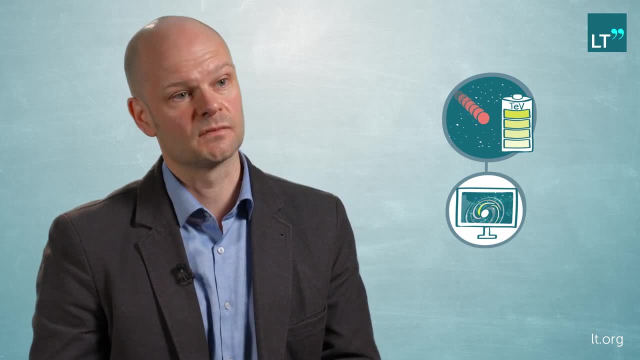 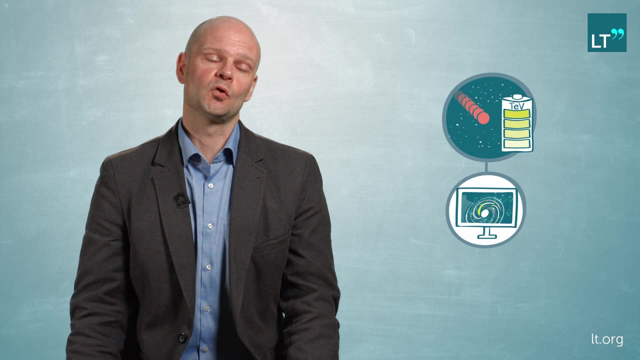 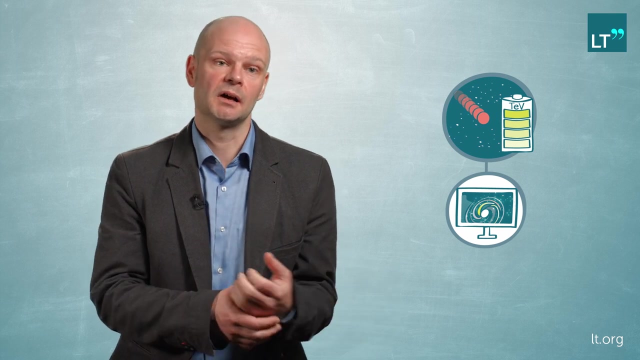 including for the first time in a self-consistent way. these relativistic particles show that galaxies look completely different if you evolve them with cosmic rays in, And also that the process of feedback on scales even of galaxy clusters we believe now may be mediated. 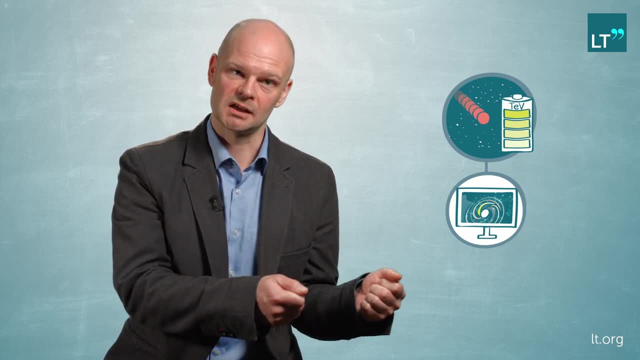 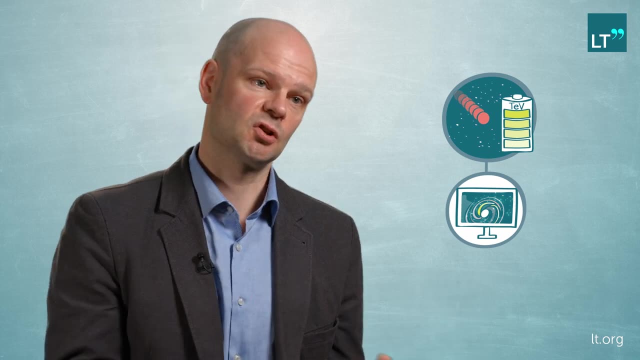 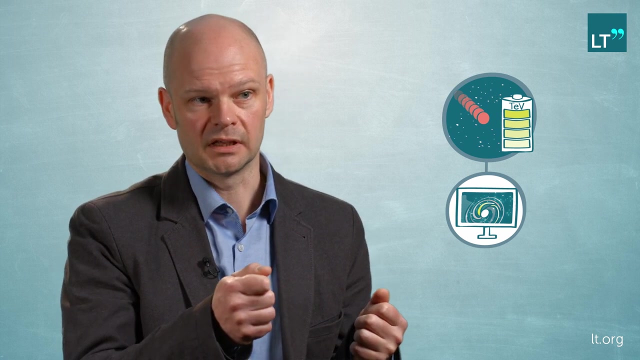 to a significant extent by these relativistic particles. So we're seeing experimental evidence there and we need more sensitive instruments, But there is a growing appreciation, I think, of the importance of these relativistic particles and of the helpfulness of these TV signatures. 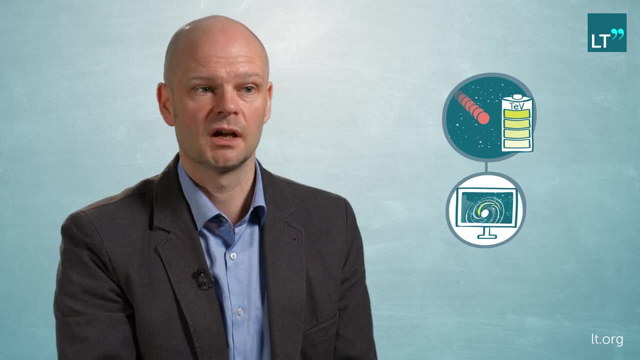 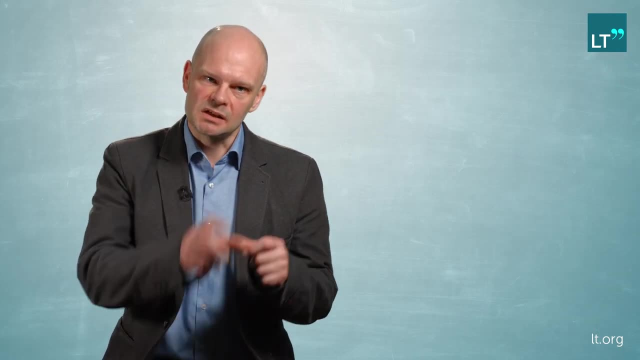 in probing these very extreme environments often and understanding where and how particle acceleration is happening to these high energies. The relevance of this is it's one piece of the jigsaw of our understanding of the universe and it's a sort of neglected piece. 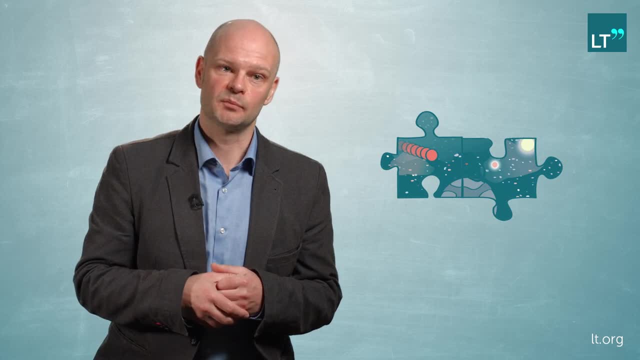 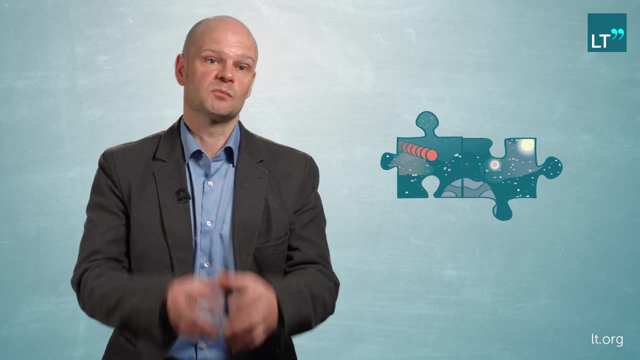 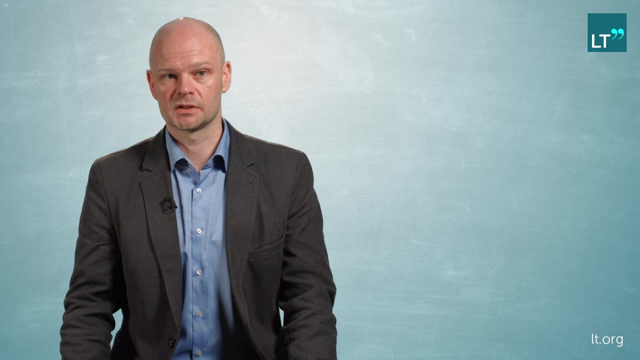 So putting this piece in has the potential to solve lots of puzzles in astronomy and also change lots of ideas about the way that many systems work or evolve and hence the impact on cosmology and the way we view the history of the universe. So, beyond understanding the impact, 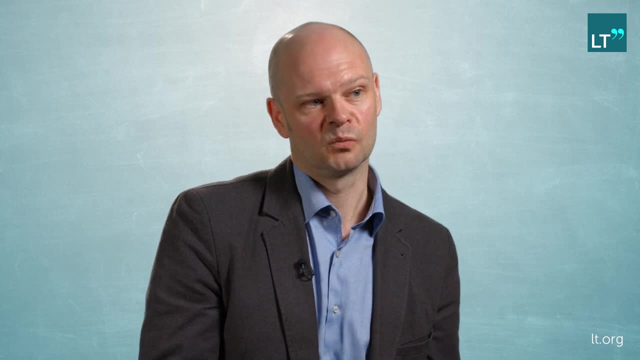 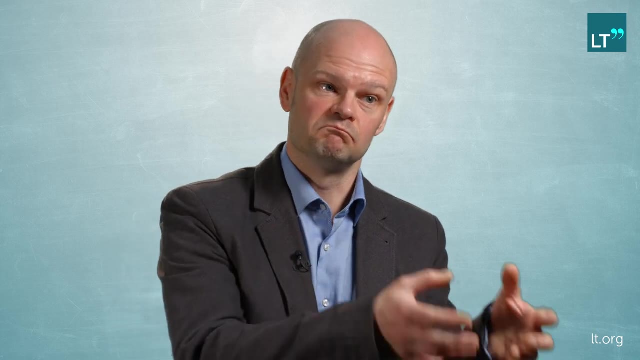 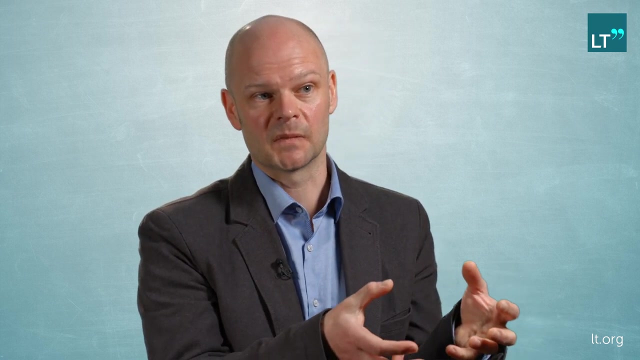 of relativistic particles, with, you know, TV photons. in the future we hope to search for the annihilation of relic particles left over from the Big Bang, so dark matter particles, And this is actually a good chance to see a gamma-ray signature of such particles. 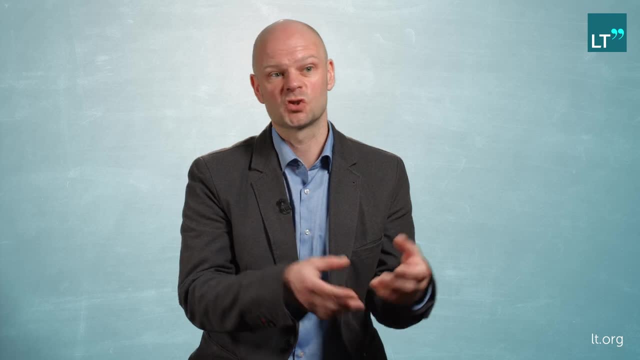 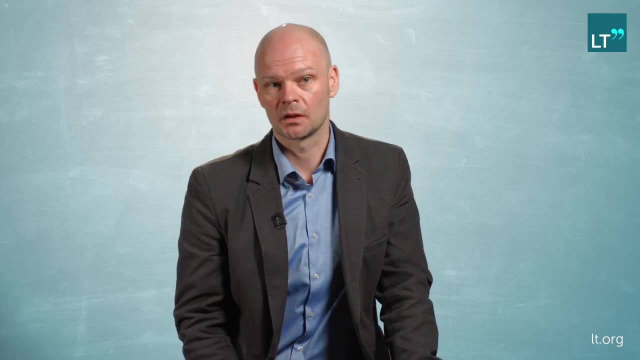 and learn about the particle nature of dark matter. We can also look for new exotic particles like axions and look for deviations from Einstein's theory of relativity that might occur because of quantum gravity effects. So because we're working with these very high-energy photons. 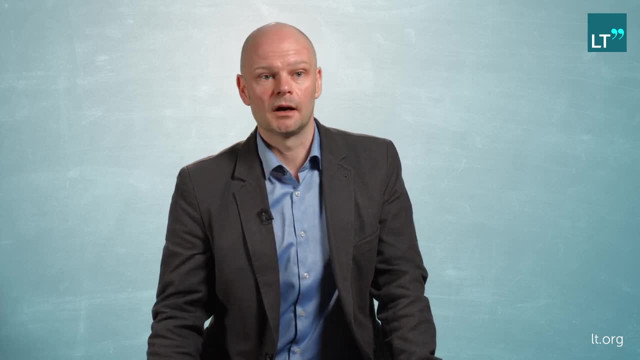 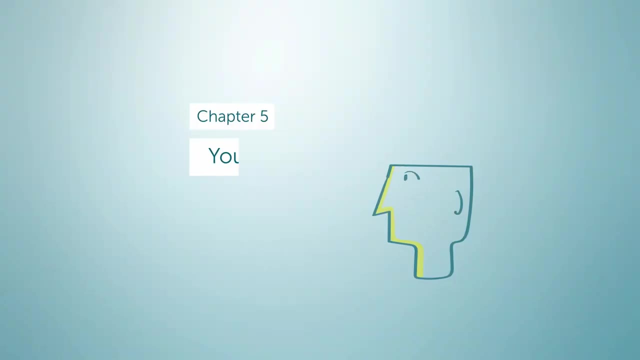 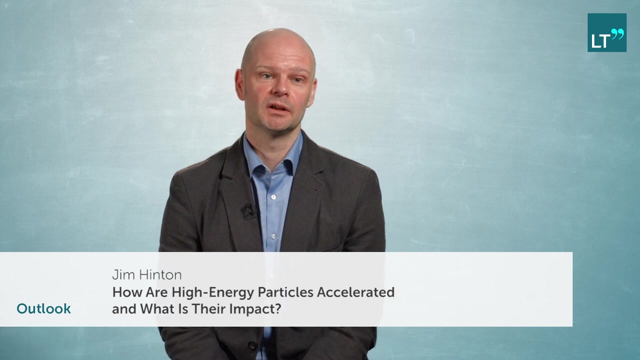 we have lots of potential to explore particle physics questions, if you like, in addition to understanding this astrophysics. So it's clear that if we want to make real progress in this field, then we need better instrumentation. We've more or less done what we can do.